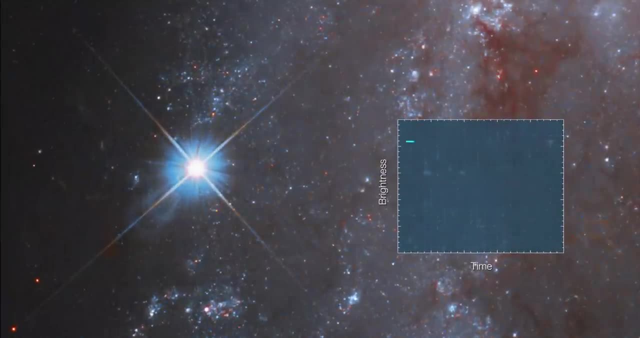 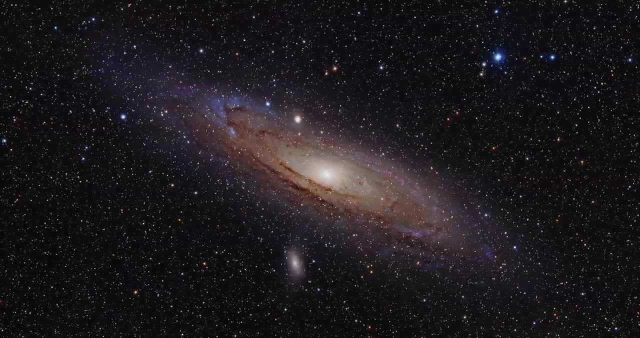 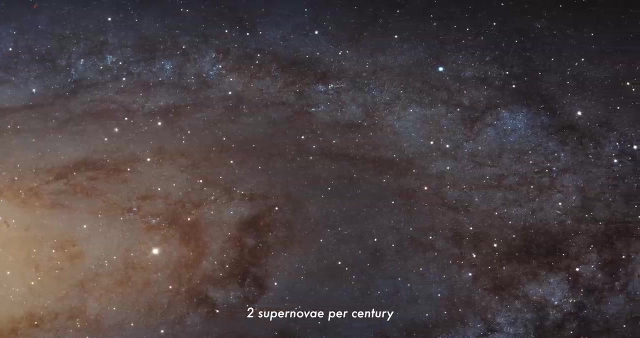 The light emitted follows a predictable pattern. It glows brightly for weeks and then fades down over a period of months. But supernovae are rare In any galaxy of 100 billion stars, or so you can expect, on average only two per century. 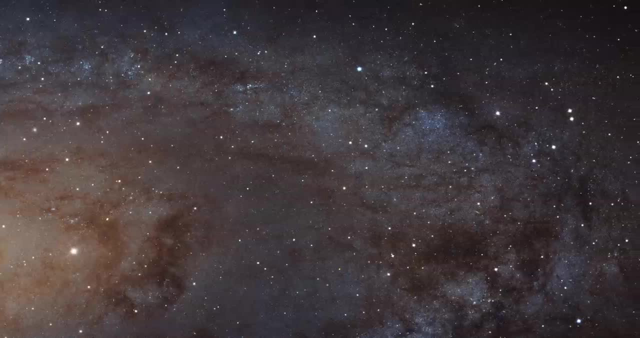 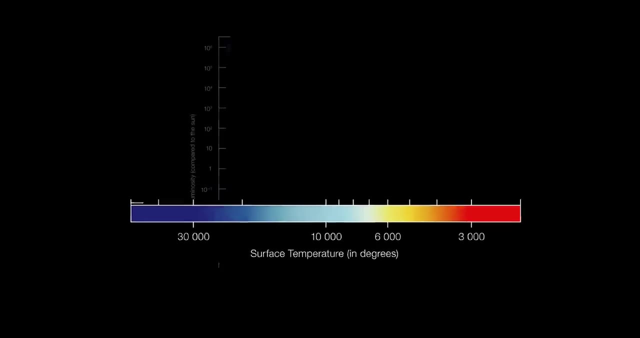 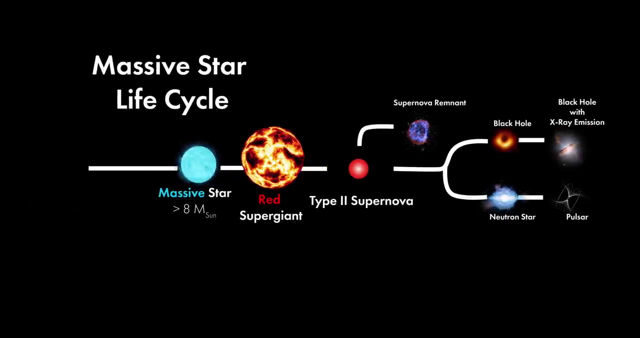 So just try picking the star that's going to explode. Now we can say how long a given star will live based on its mass, luminosity and color temperature. These data pinpoint its stage of life, But the estimate of exactly when a large star will go supernova has big error bars. 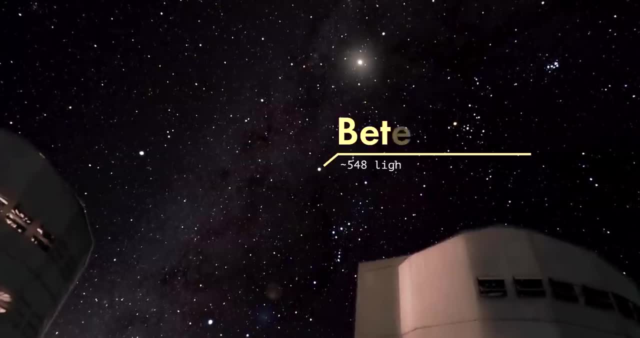 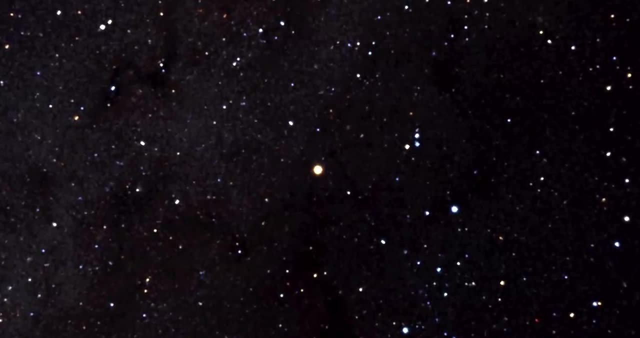 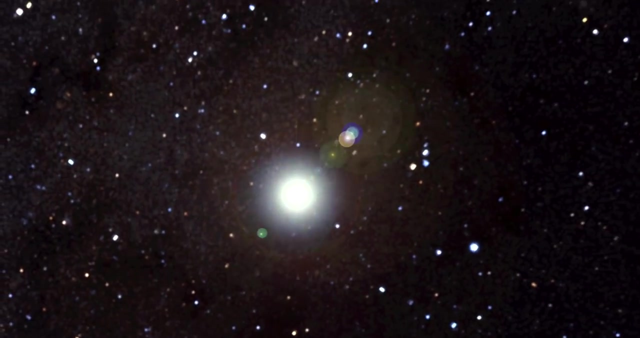 Take the red supergiant Betelgeuse, for example, in our own Milky Way galaxy. It is a great candidate to go supernova. Scientists think Betelgeuse will explode any day now in the next few hundred thousand years. When it does, it'll be so bright you can see it in the daytime. And it will rival the full moon's brightness at night. So what's the difference? According to the lifespan of a star, 100,000 years is a brief window of time, But for us short-lived humans, it may as well be forever. 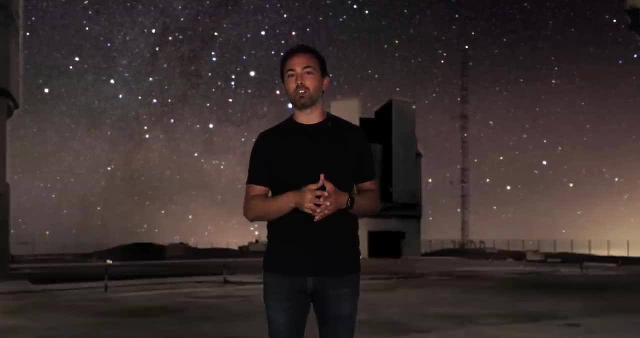 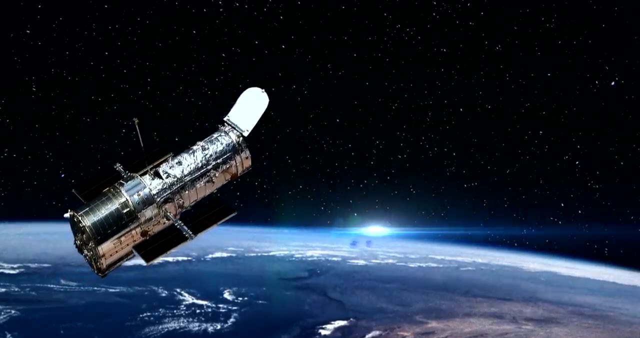 So you might think it would have been a tough sell when the scientists who predicted we'd see a supernova in November 2015 asked for time on the Hubble Space Telescope to take pictures of Galaxy SP 1149. But their request was granted. 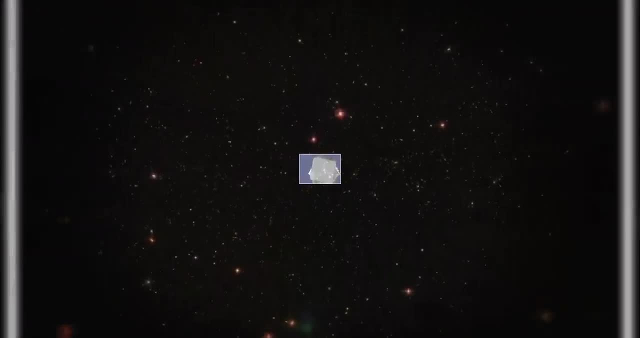 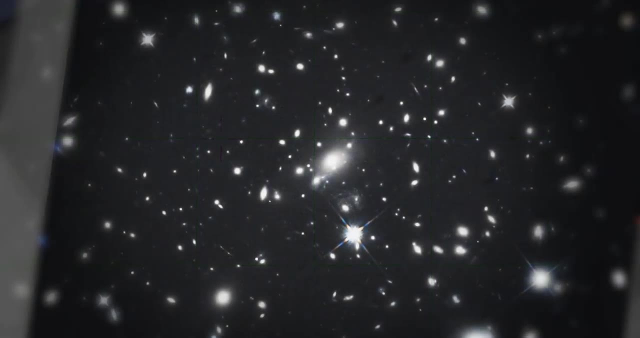 They could image this part of the sky roughly once a month, starting on October 30th, But they couldn't Before this. the galaxy was too close to the Sun to point Hubble at it. In this first image, taken at the end of October, there is no supernova. 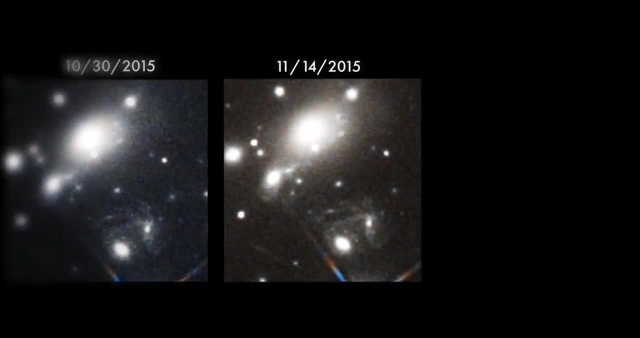 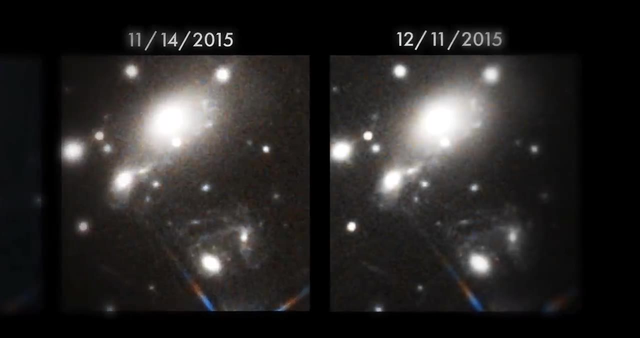 The next image was taken on November 14th- Again no supernova. But in the third image, taken on December 11th- jackpot- There's a supernova, right where they predicted it would be and almost exactly when they said it would happen. 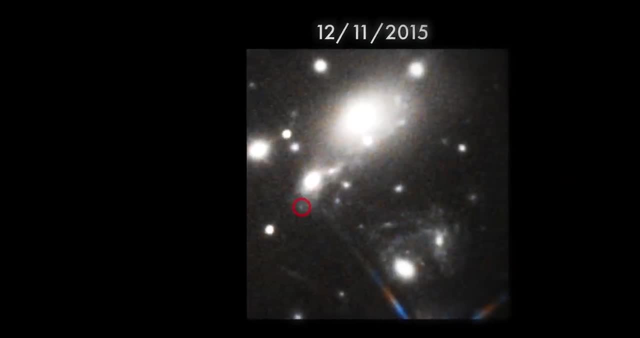 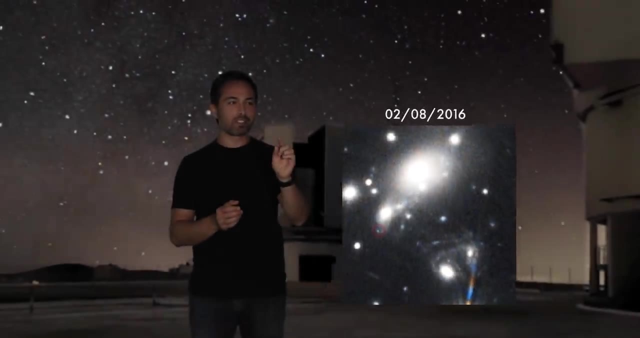 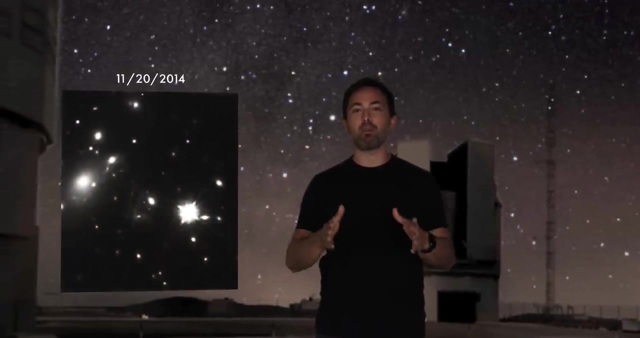 So how did they manage to predict a supernova almost to the month? Well, the truth is, they had seen this same exact supernova before, Not once, not twice, but four additional times. A year earlier and five months before the predictions, Hubble took this image. 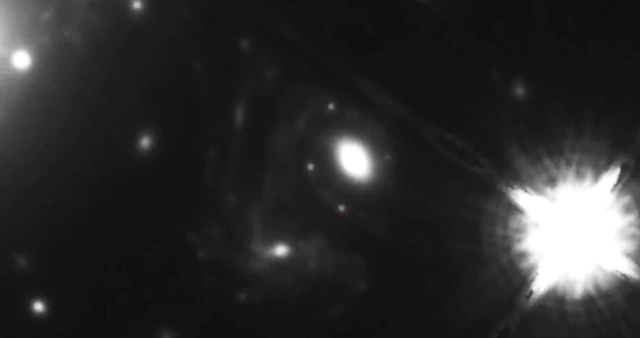 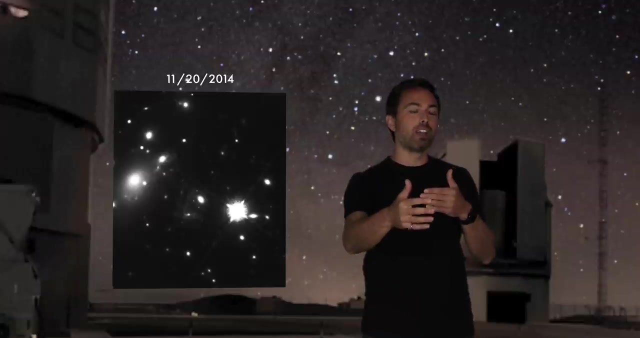 See those four bright dots. Those are multiple images of that same supernova. The reason we see the same supernova in four different locations is because there is a lens between us and the exploding star- Not a lens made of glass, of course. 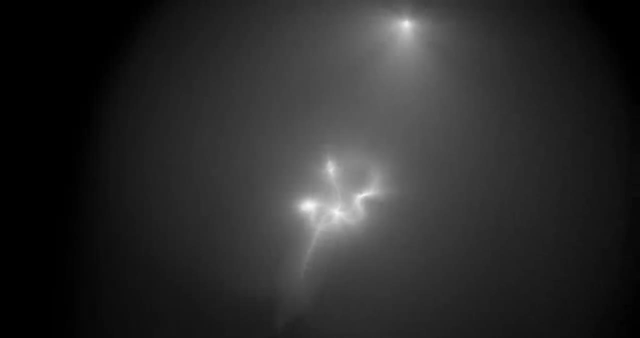 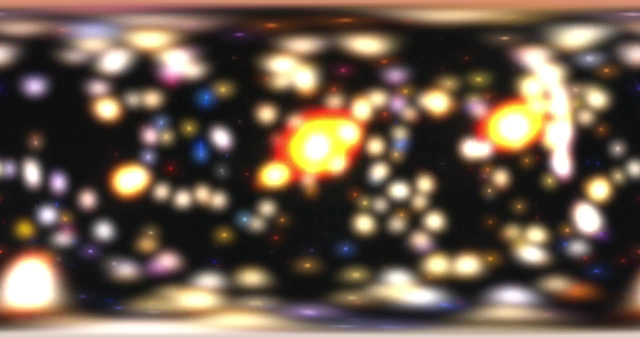 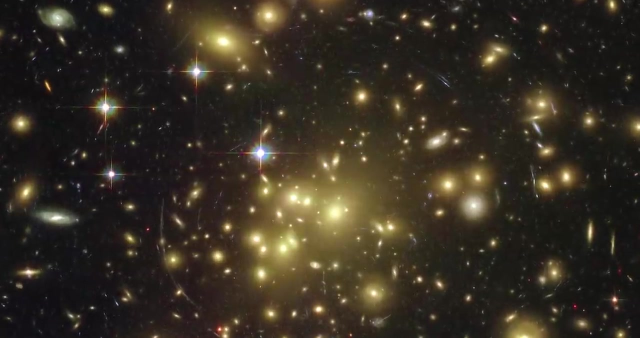 But a gravitational lens made of a huge amount of ordinary matter and dark matter. Gravitational lensing tends to magnify distant sources and increase their apparent brightness as rays of light become concentrated. This smears the image of distant galaxies into arcs, strands and all kinds of weird. 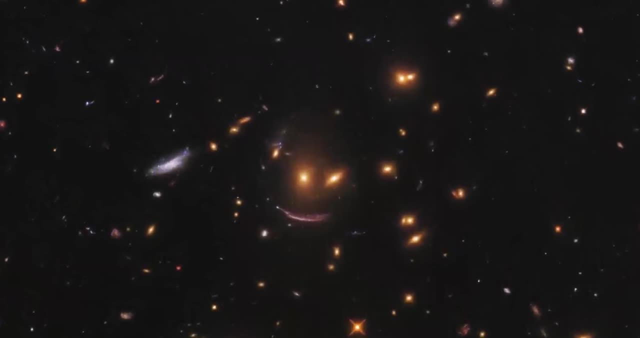 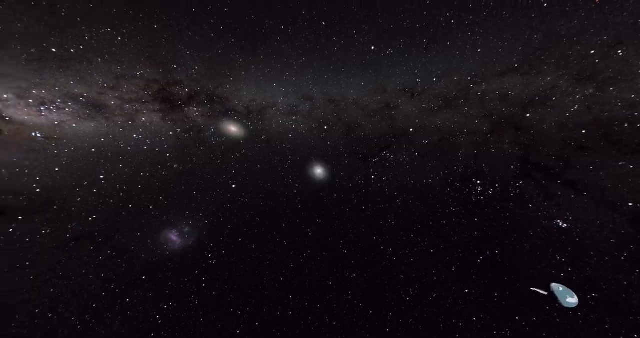 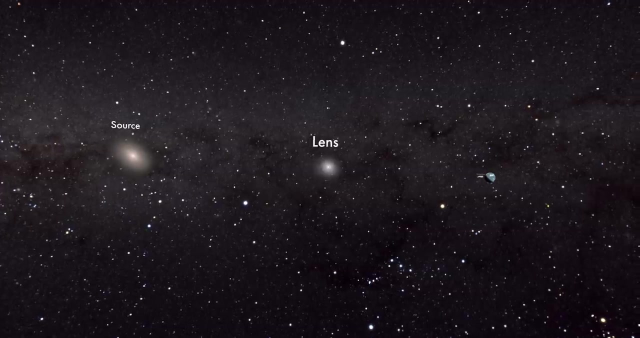 shapes And, of course, to some distant observer in another galaxy. the light from our own Sun and Milky Way galaxy may be similarly warped. In gravitational lensing There are three essential components: The source, the lens and the telescope. If the lens and the source are spherically symmetric and if the source lens and telescope, 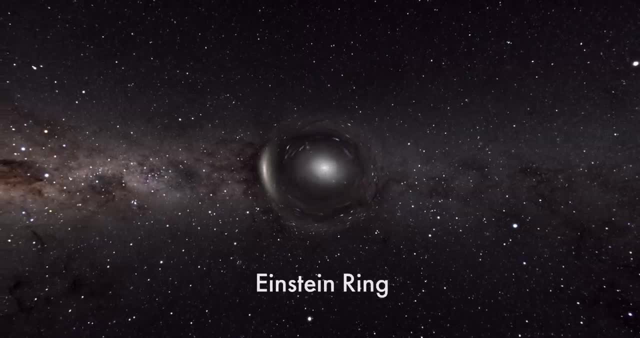 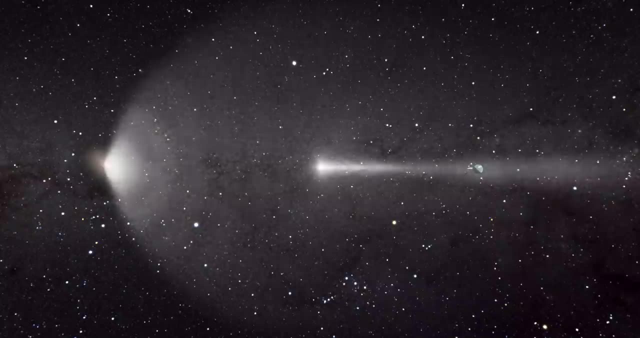 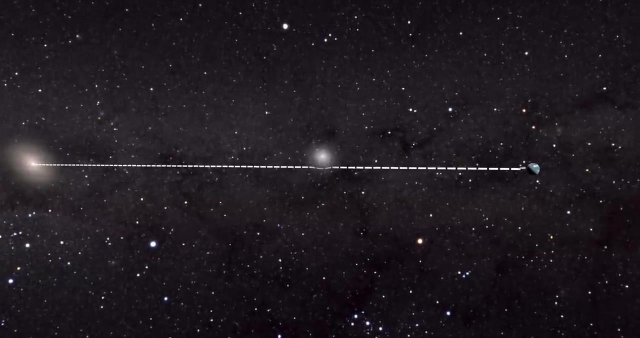 are perfectly aligned, you get what's known as an Einstein ring. The light from the source is bent around the lens equally in all directions, leading to the image of a smeared out ring If the source and the lens are spherically symmetric but are not perfectly aligned. 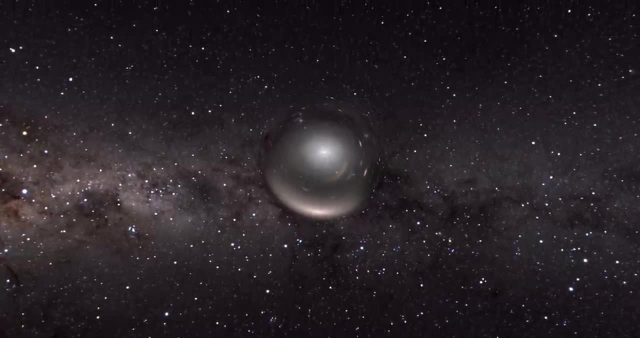 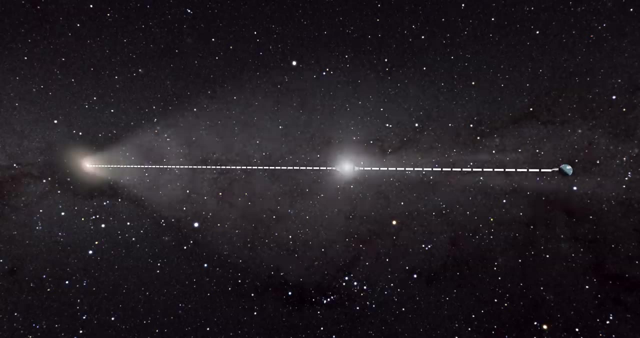 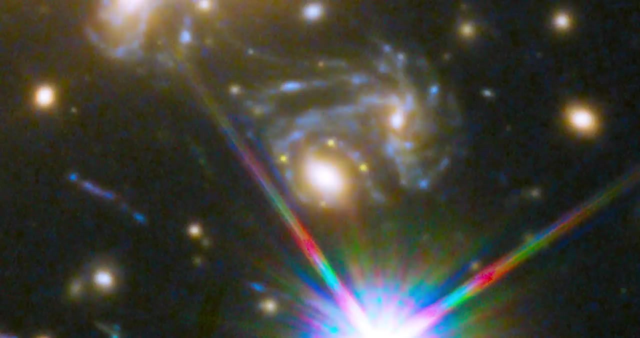 then what we end up seeing is a sphere. And if the source, lens and telescope are aligned, but the lens is not axially symmetric, for example, it could have an elliptical shape. well then you get four images in the shape of a cross. 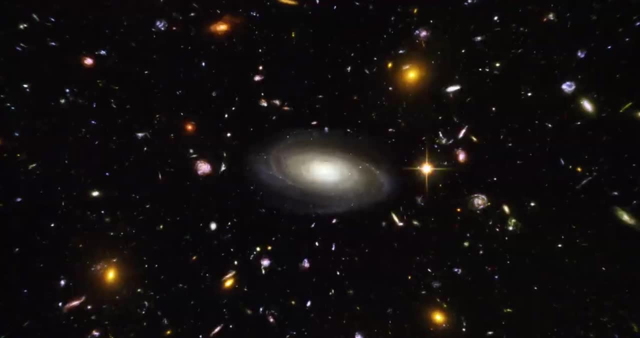 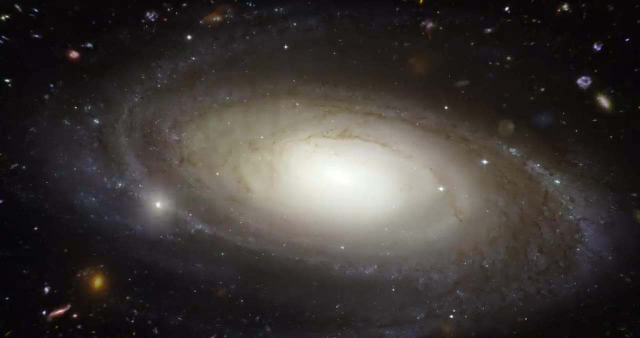 An Einstein cross. So what happened with our supernova is: 9.3 billion years ago, a dying star in a galaxy far, far away went out with a bang As a supernova. The explosion sent out a blast of light in all directions. 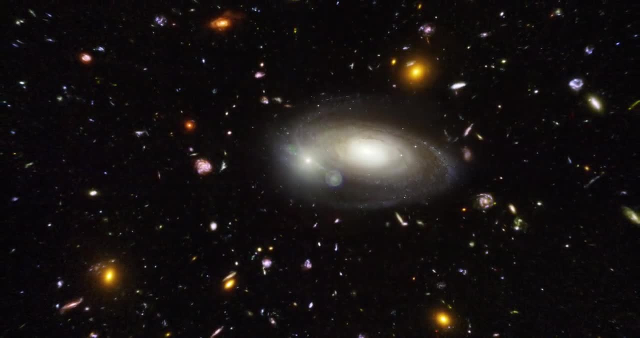 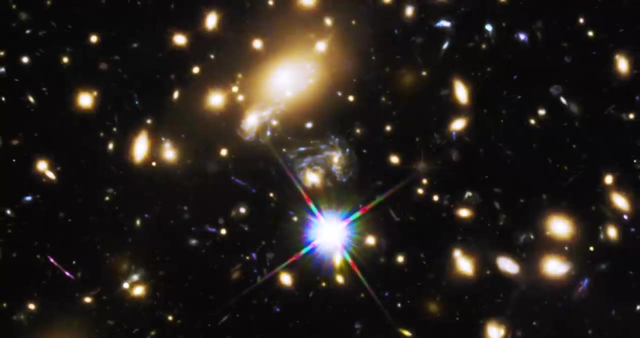 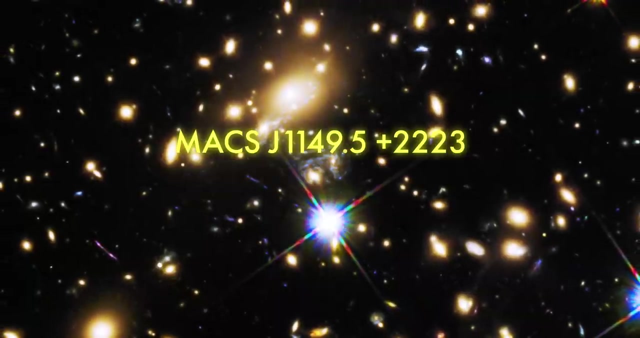 About 5 billion years ago, before the earth even existed, that light encountered a very massive object that warped space time. It was a cluster of galaxies called MACS J1149.5 plus 2223.. Yeah, I know that's a mouthful, but the name just tells us where in the sky it was discovered. 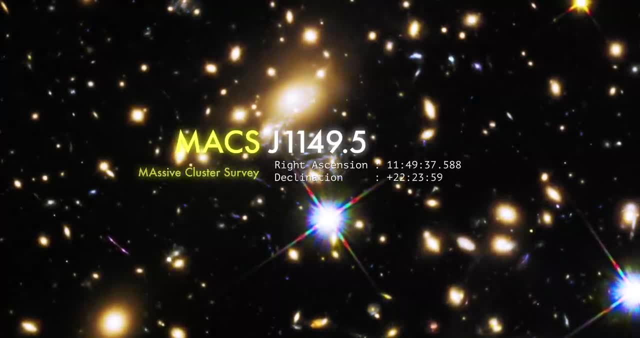 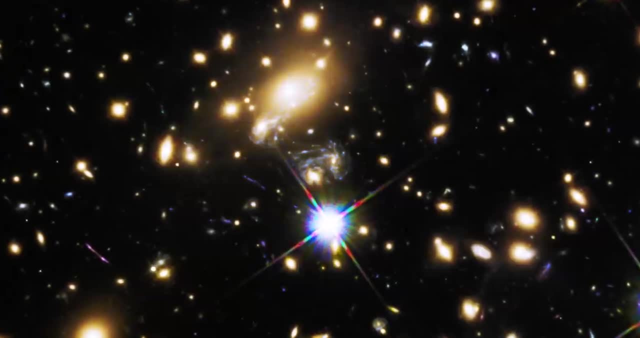 by the Massive Cluster Survey. What is a galaxy cluster? What is a galaxy cluster? A galaxy cluster is made up of lots of massive substructures like individual galaxies and halos of dark matter. At some point as the light traveled through this region, it encountered an elliptical 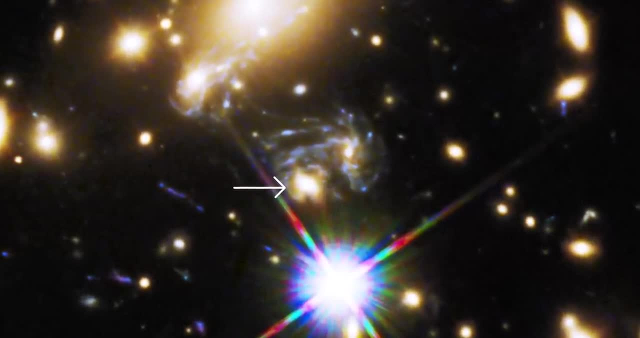 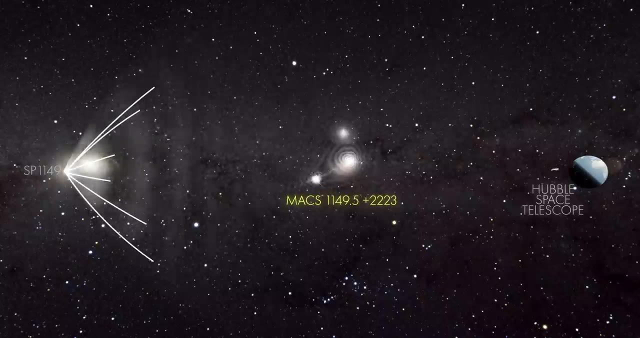 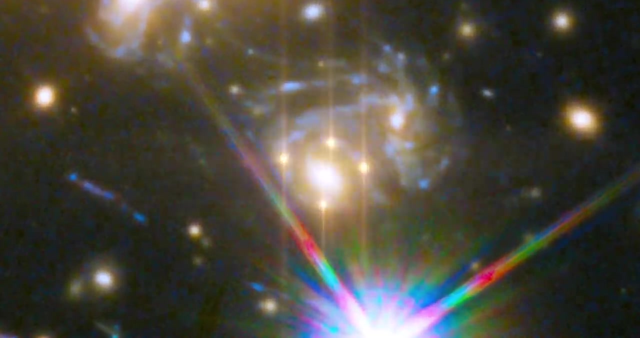 galaxy almost perfectly lined up with where the earth would eventually be, And the gravitational deflection focused light rays that were initially diverging onto paths that converged at the earth. This is why we saw the same supernova in four different locations. Not only did the supernova appear at four different places, the images also appeared. 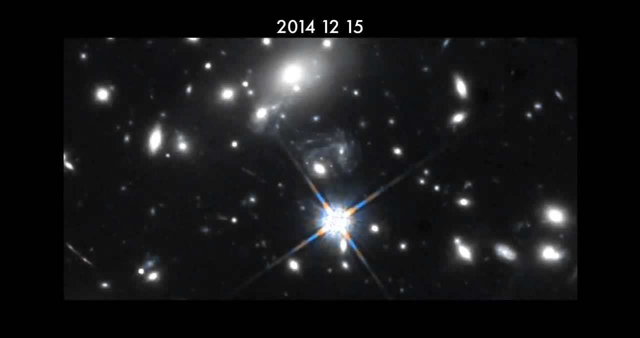 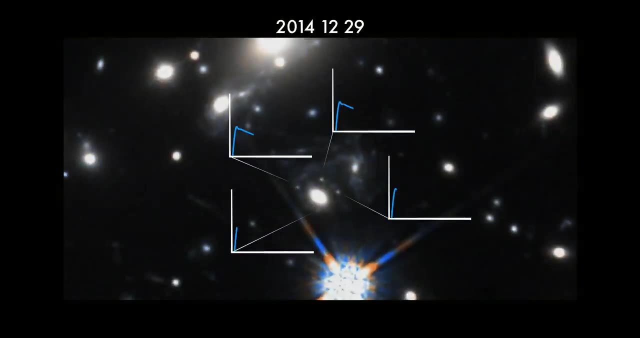 at different times. Relative to the first image, the others were delayed by periods ranging from five days to over three weeks, And we could measure this time delay because of the distinctive light curve of the supernova. Some of the images of the explosion were further along in their light curve than others. 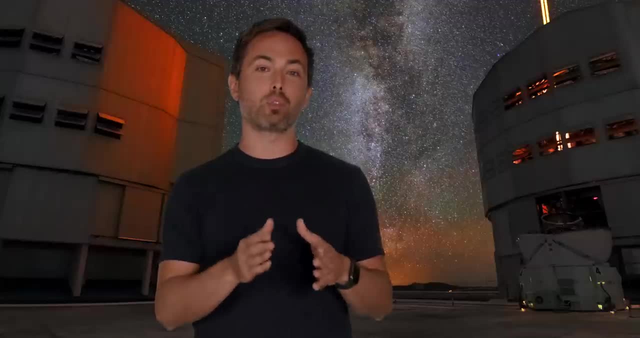 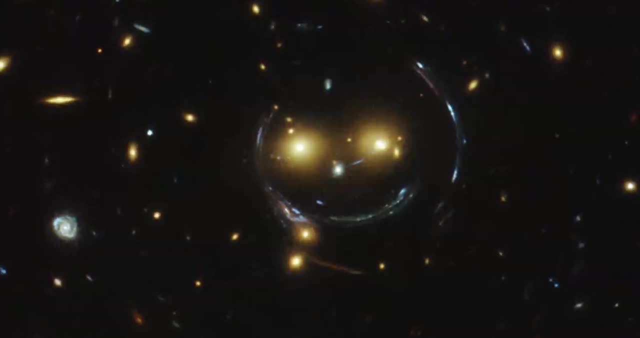 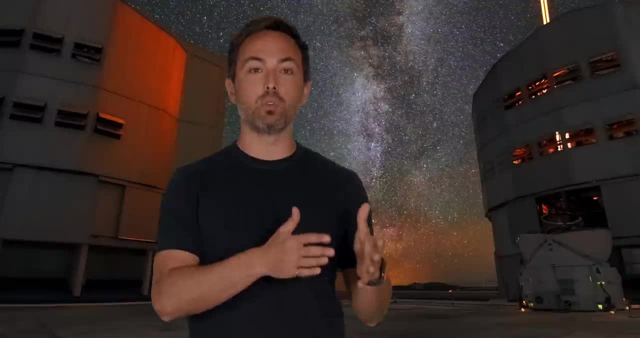 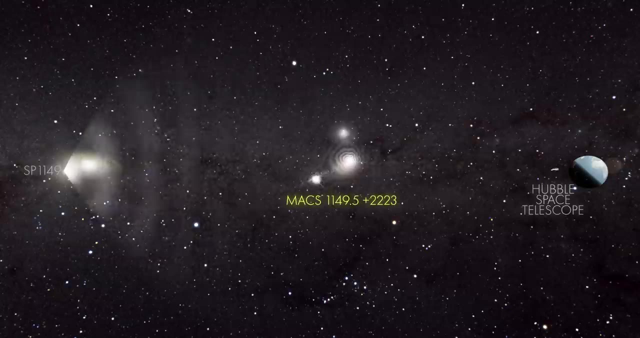 But these objects don't change predictably with time, so there's no way to use their images to work out the relative time delay between them. Now, one reason for the time delay between the supernova images is because the four paths the light took were different lengths. 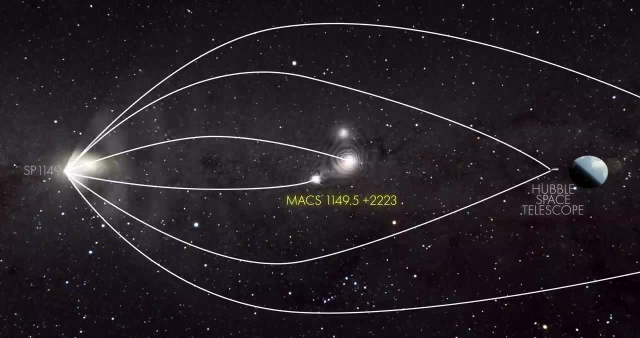 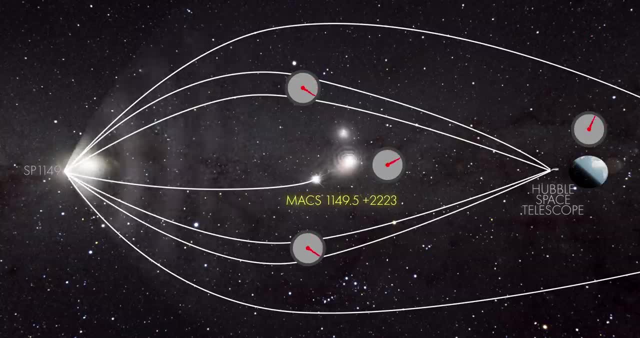 So it just took the light longer to travel further. But there is another reason, Which is that light passing through curved spacetime appears to travel more slowly relative to an external observer. This is much less intuitive, but it's a well-established and well-tested part of general relativity. 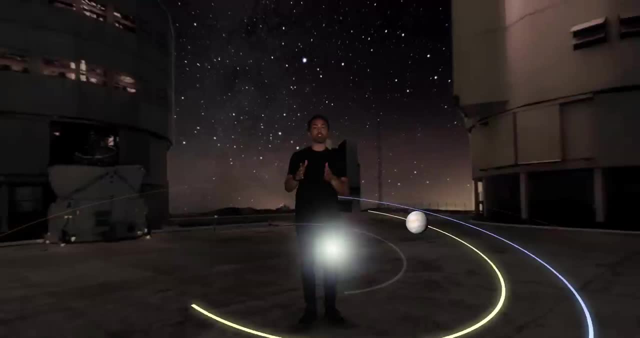 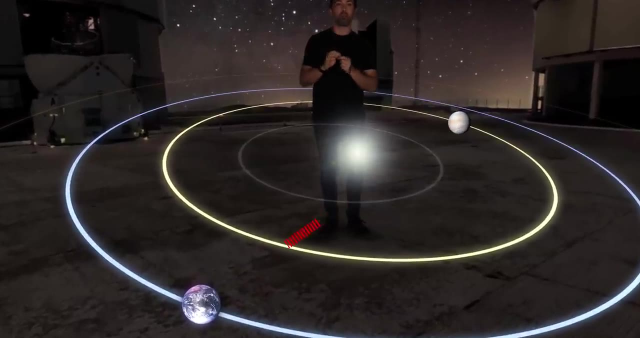 Back in 1964, Erwin Shapiro suggested it would be possible to test this gravitational time delay by sending radar signals to Venus and measuring how long it takes for the echo to come back. He calculated that, due to the gravitational influence of the Sun, the signals would take 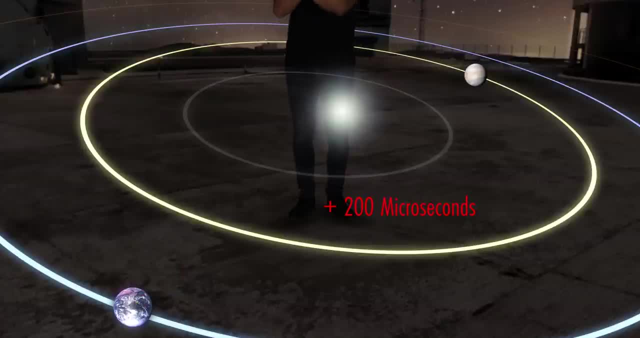 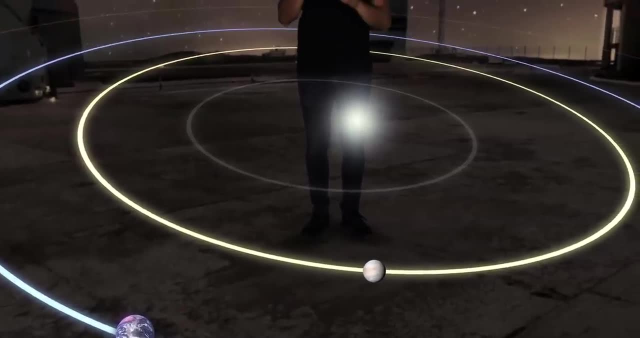 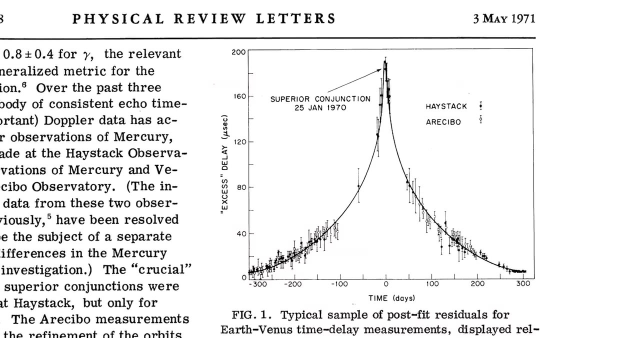 an extra 200 microseconds when Venus was on the other side of the Sun compared to when it was close to us. This is solely a gravitational time delay, not related to the extra distance the light has to travel, And within a couple years, experimental data revealed the gravitational time delay for 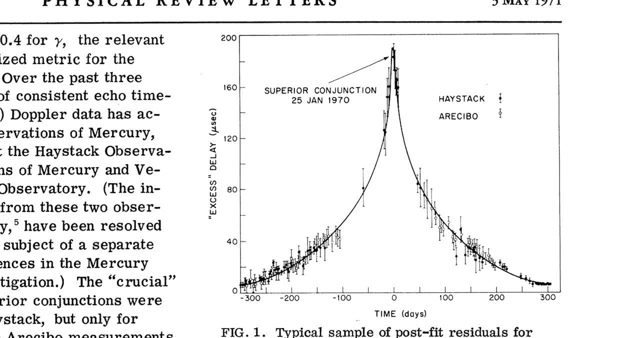 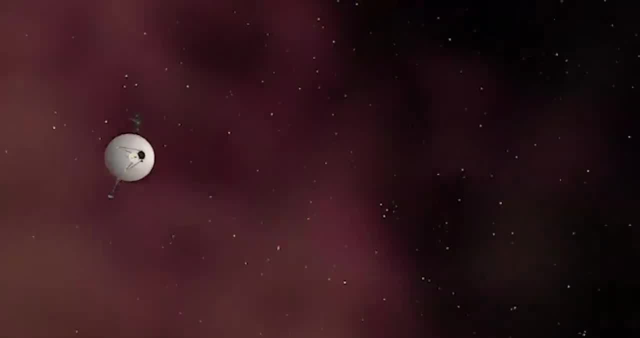 light traveling past the Sun was exactly as predicted Today. in order to accurately determine the distance to the Voyager and Pioneer spacecraft, this Shapiro time delay must be taken. Now I want you to have a look at the four supernova images again. 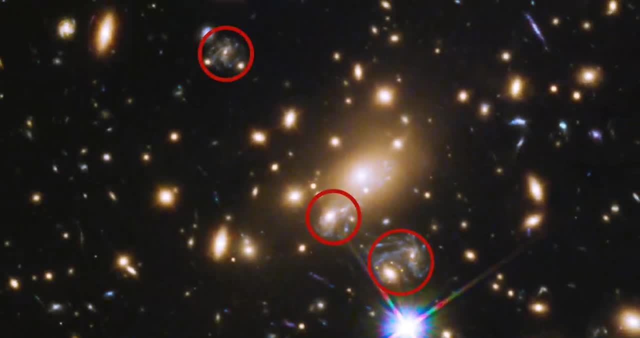 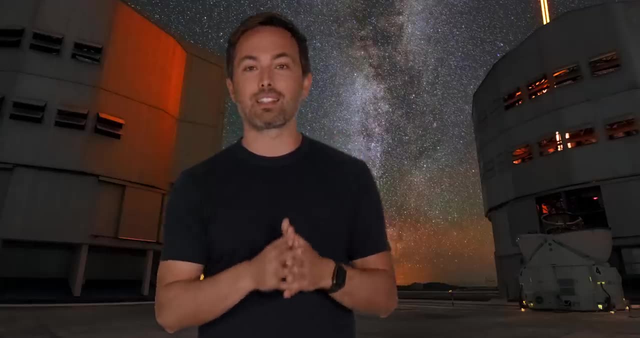 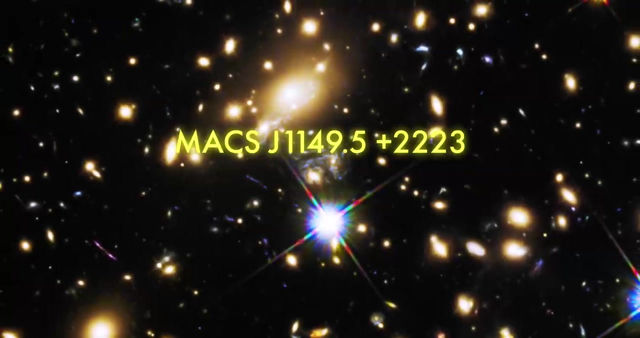 Do you notice how the same galaxy appears three times in this image? That is the supernova's host galaxy. It is itself lensed by the massive galaxy cluster MACS J1149.5 plus 2223.. In fact, this cluster lenses tens of galaxies, so scientists had been studying and modeling. 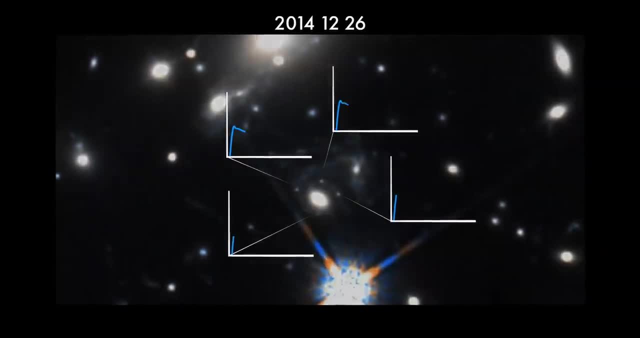 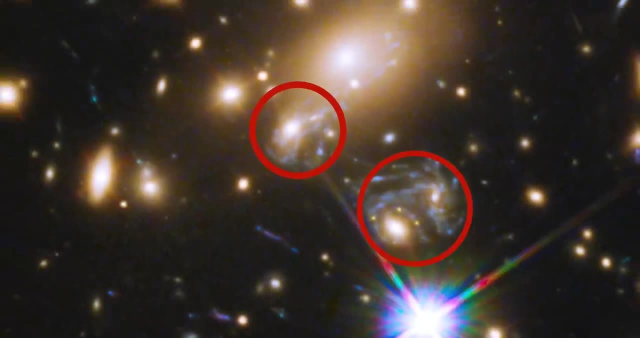 the distribution of matter in the galaxy And they found that the supernova would appear in the cluster long before the supernova. They asked: if we see these four images of the supernova in one image of its host galaxy, when would the supernova appear in these other two images of the host galaxy? 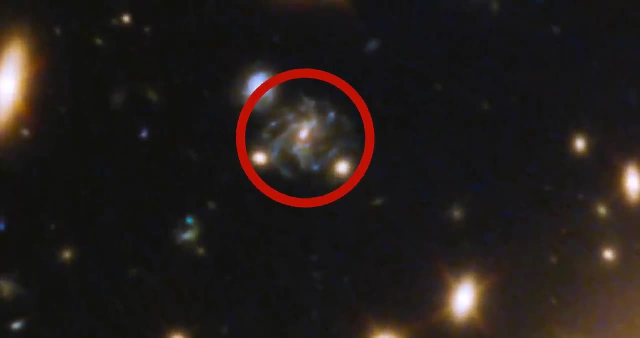 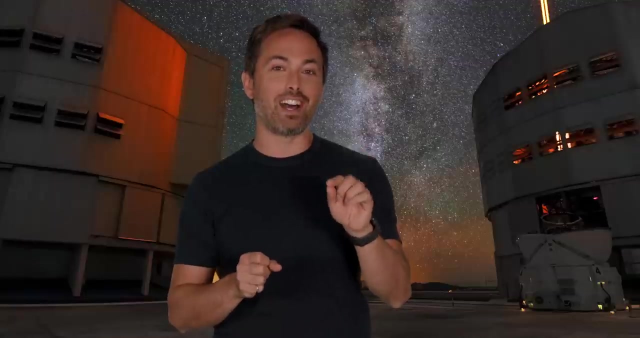 And using the models of mass distribution and general relativity, they calculated that in this image the supernova would have appeared 20 years earlier, in 1995.. Now there are no close-up pictures of this part of the sky from 1995, so there is no. 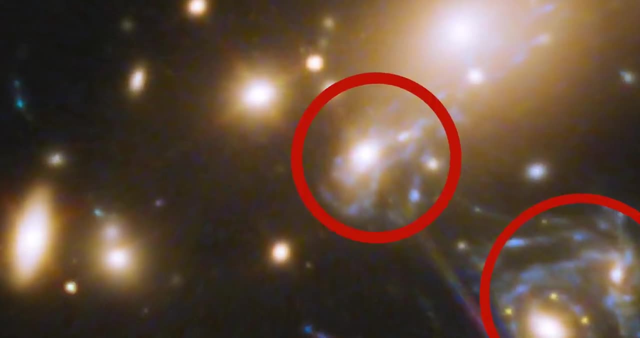 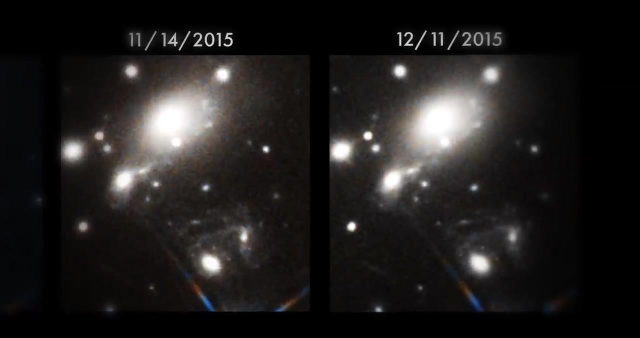 way to check. But in the other image of the galaxy they predicted the supernova would appear again in about one year's time, almost exactly when it showed up in that Hubble image. This successful prediction is a fantastic confirmation of our understanding of light. 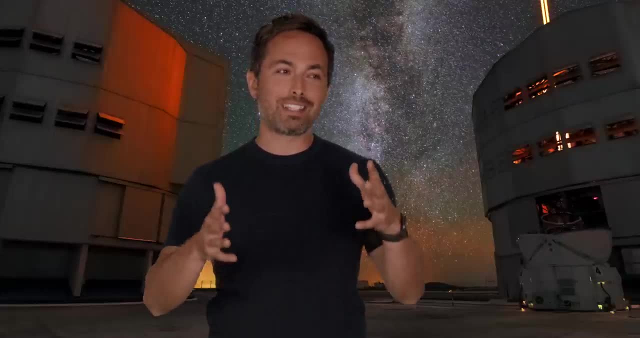 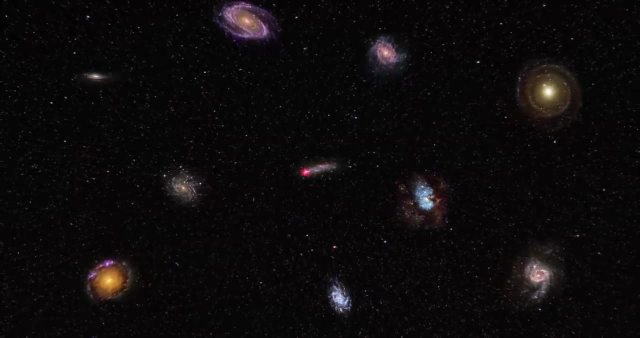 and gravity on the scale of the whole universe. But it has even bigger implications. One of the hottest debates in astronomy right now is: how fast is our universe actually expanding, Measured by the Hubble constant, the rate at which distant galaxies are receding away? 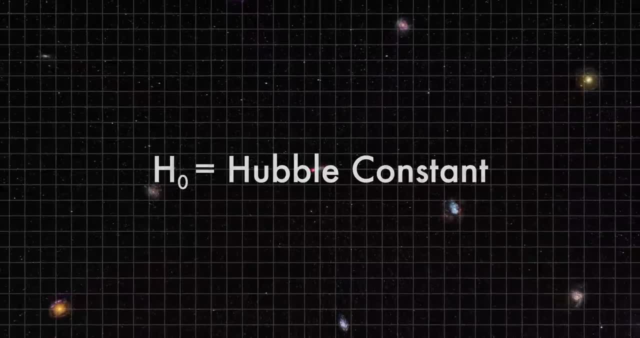 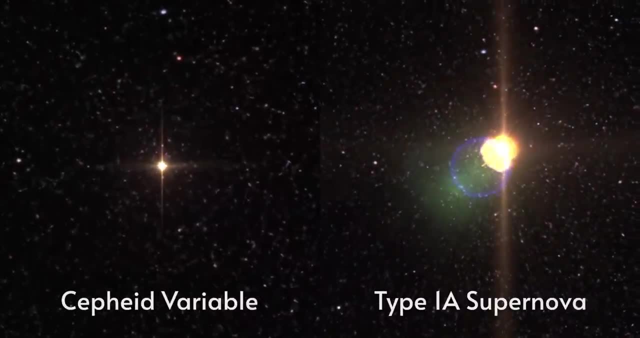 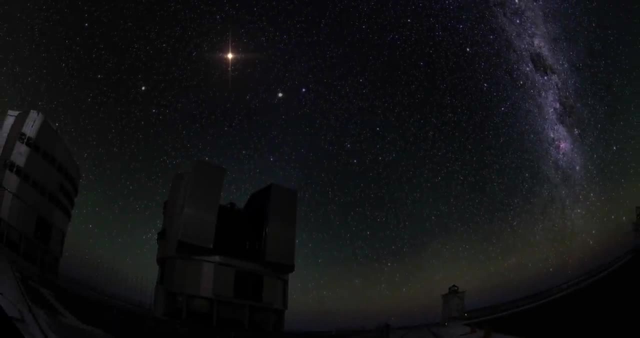 from each other, depending on their distance apart. Now there are two main ways this measurement has traditionally been made. One is to look for stars in the nearby universe whose absolute luminosity we know. Then we can use how bright they appear to us to determine how far away they are. 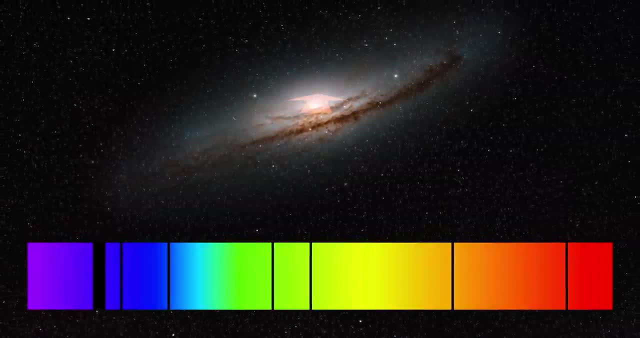 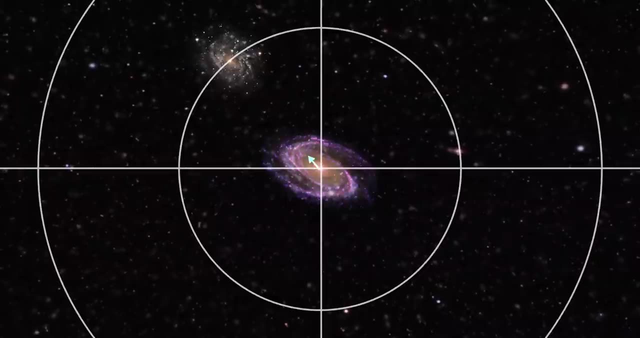 If you combine this distance information with how redshifted their light is, you can work out how fast the universe is expanding. This is known as the distance ladder method, And the value of the Hubble constant it produces is around 74 kilometers per second per megaparsec. 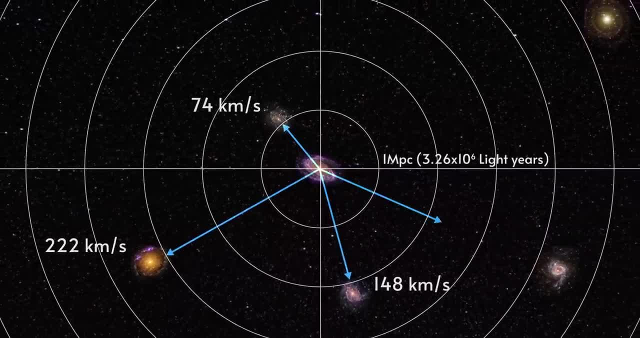 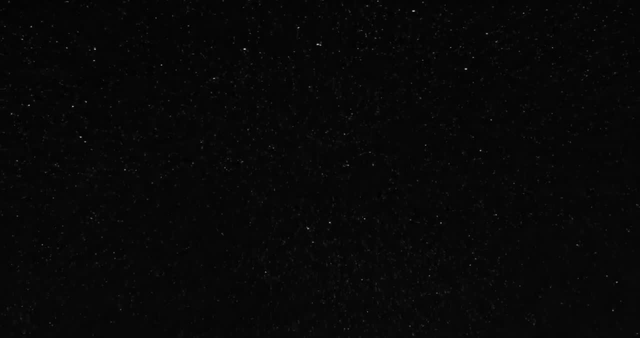 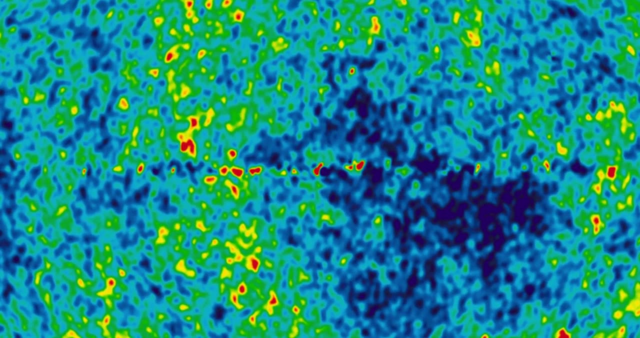 Meaning for every megaparsec that separates two galaxies. they will, on average, be moving apart at 74 kilometers per second. The other way to measure the Hubble constant is to study the features in the cosmic microwave background radiation, which is essentially just a picture of the early universe. 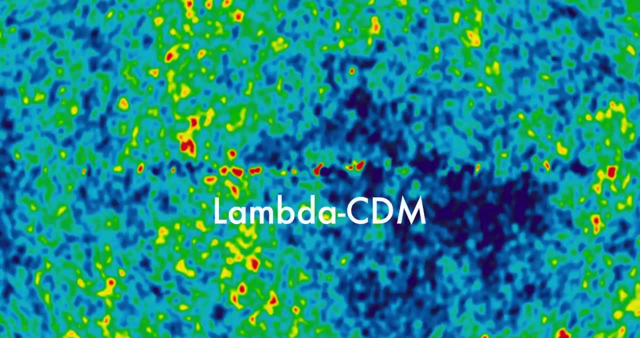 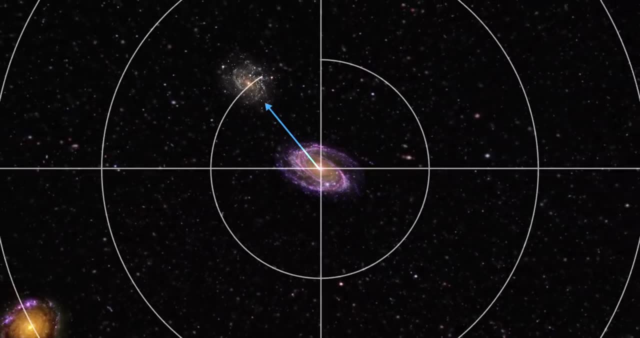 Using the standard model of cosmology, Which is the first one, Which is called Lambda CDM, We can work out how this early universe picture would expand over time. The result obtained from this method comes out to 67 kilometers per second, per megaparsec. 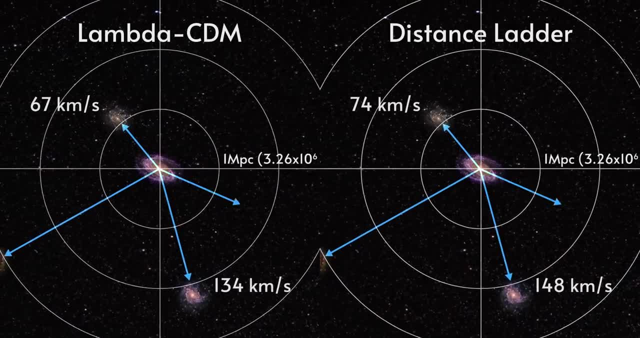 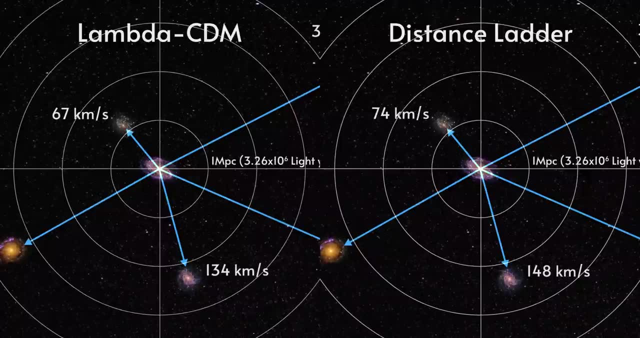 Substantially slower than the 74 found via the other method. Now, over the years, both of these techniques have been refined, reducing their uncertainties, But the values have not gotten closer together. So at this moment, the two values really seem different. 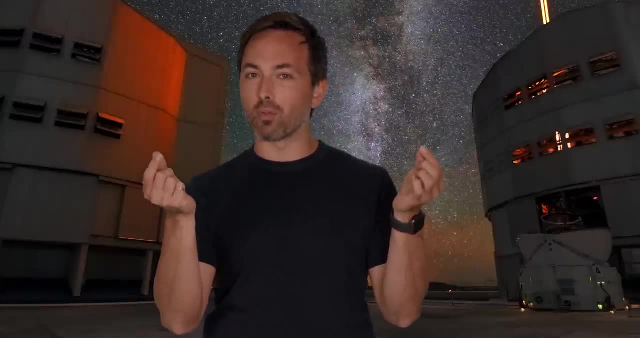 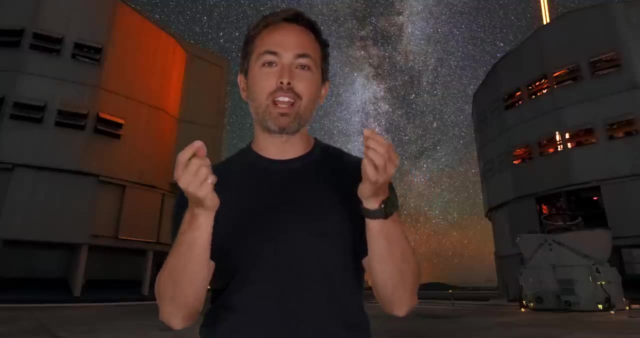 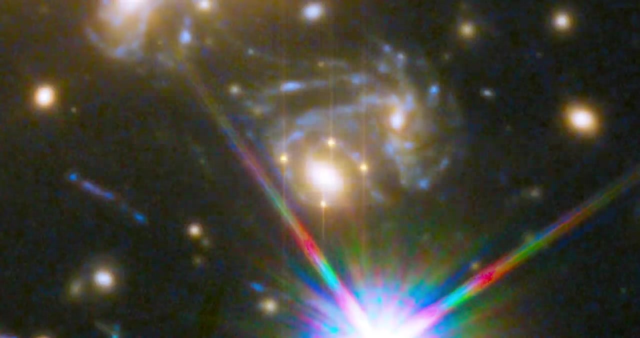 They are on the cusp- On the cusp of being a 5-sigma result. Astrophysicist Joseph Silk has called it a possible crisis for cosmology. But there are independent ways to measure the Hubble constant, And one of them is to look at a multiply lensed supernova and use the time delay between their 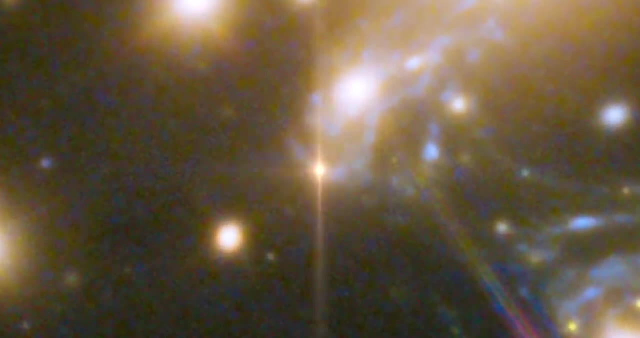 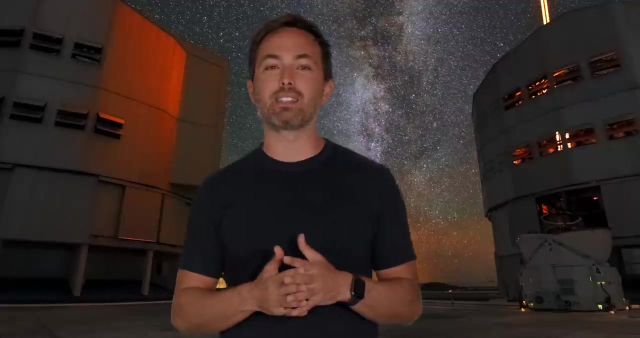 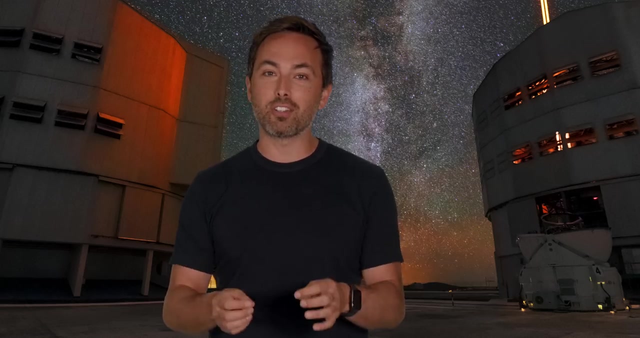 appearances to work it out. This was first proposed by a Norwegian astronomer, Sjur Refsdal, in 1964.. Since this is the first observed multiply lensed supernova, it has become known as supernovae. Calculations of the Hubble constant. from this data yield a value of 64 kilometers per second, per megaparsec. 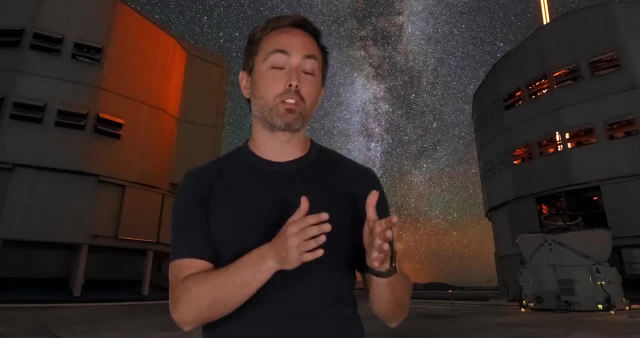 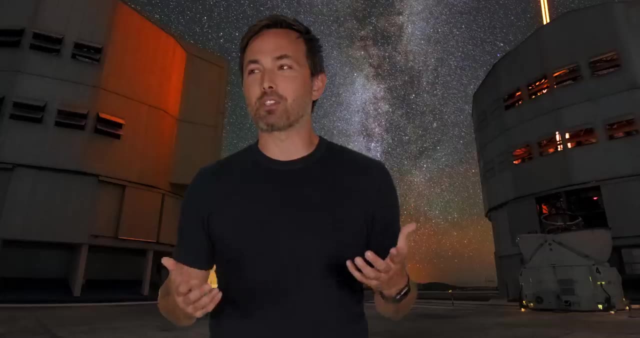 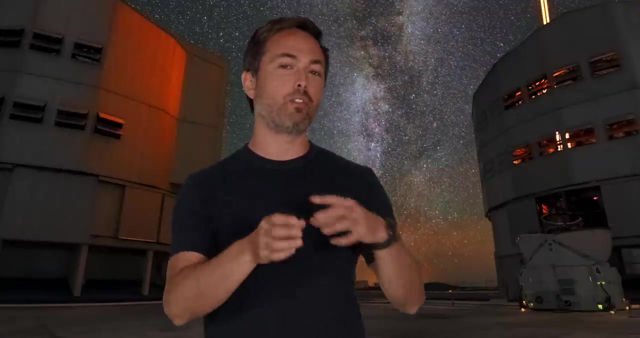 Although that result has large error bars, it is more in line with the measurements of the cosmic microwave background radiation than with the distance ladder method. The thing I keep thinking about is how strange space is. I used to think of it essentially like glass: fundamentally transparent, with some foggy. 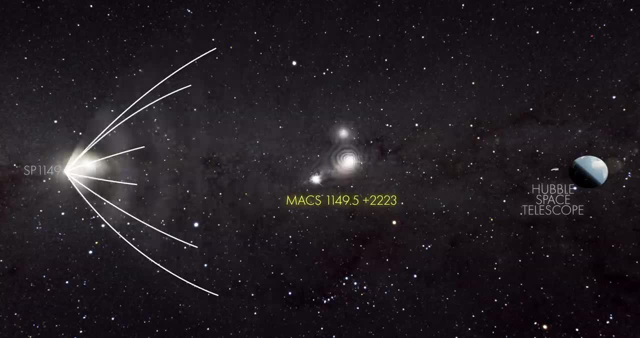 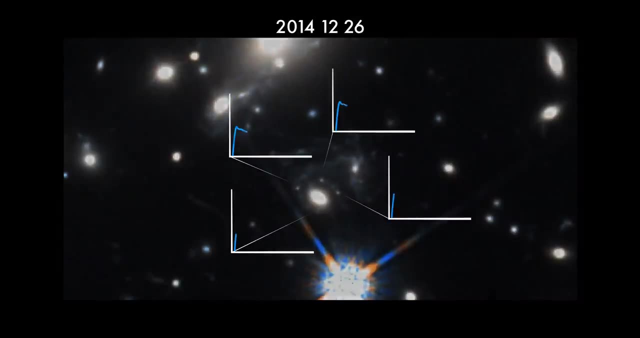 regions or slight distortions. But here we have space that is not transparent Space, warping light on multiple curved trajectories, making the same event appear in six different places on the sky, separated by days, weeks, a year and 20 years. 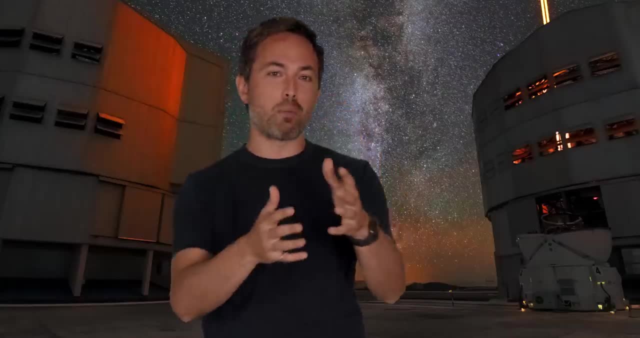 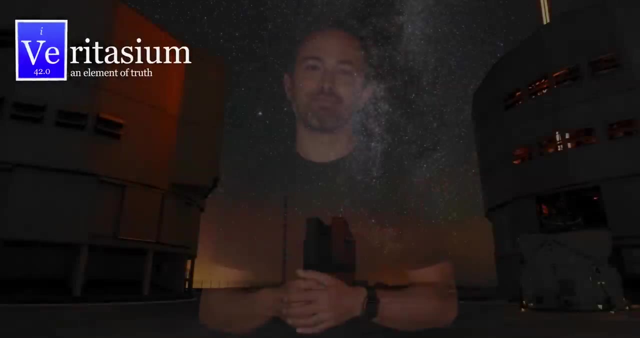 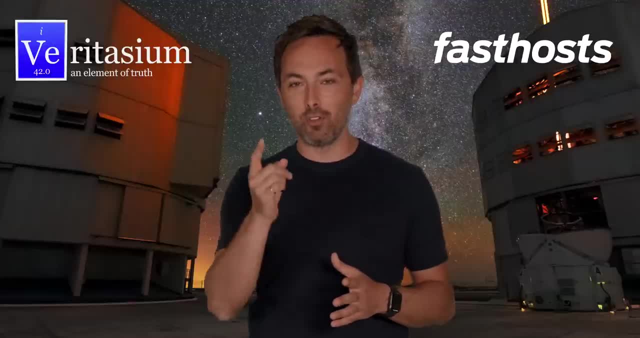 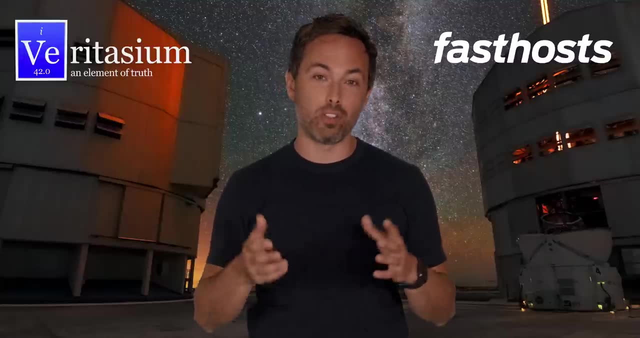 You can win a $5,000 tech bundle, including your dream PC setup, if you can answer my techie test question Now. Fasthosts provides a wide range of web hosting products. If you're in the UK and you're looking to start a podcast or a blog or a business, you're. 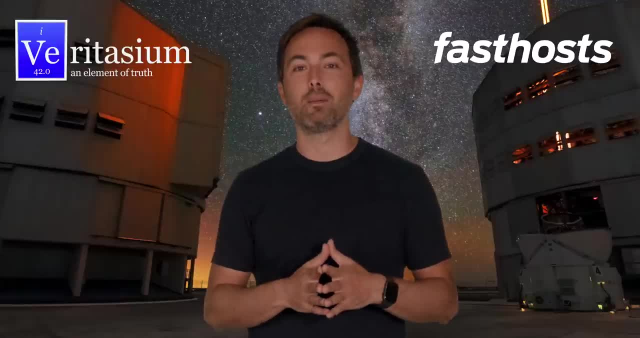 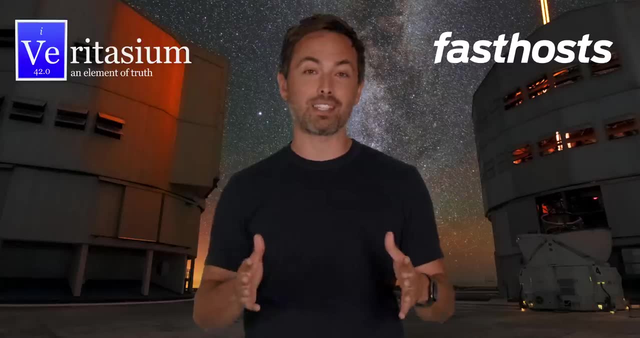 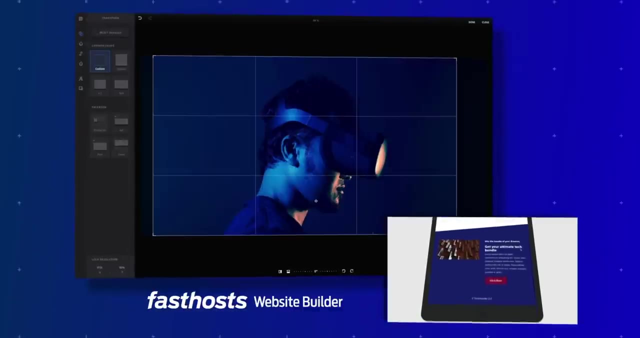 going to need a website, And Fasthosts have got you covered. They offer easy registration for a huge range of domain names, with powerful management features included. Plus, they have a website builder with drag and drop templates, Custom mobile optimized website with no coding required. 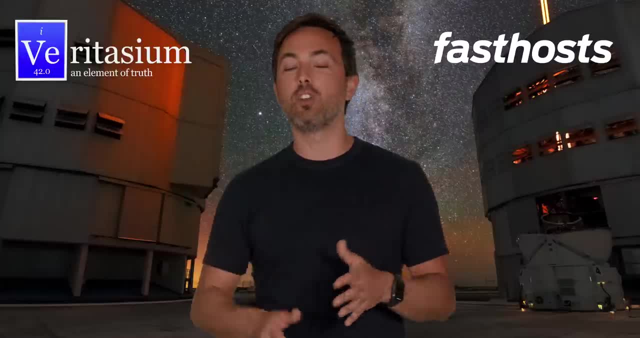 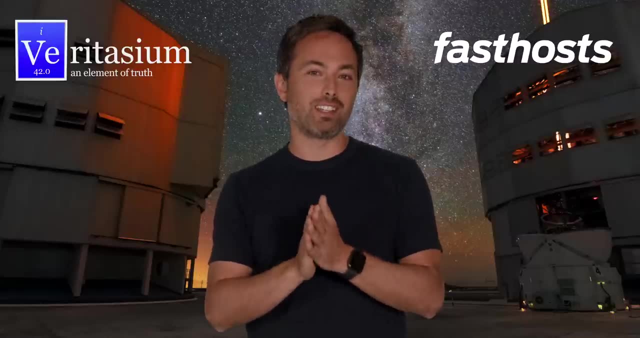 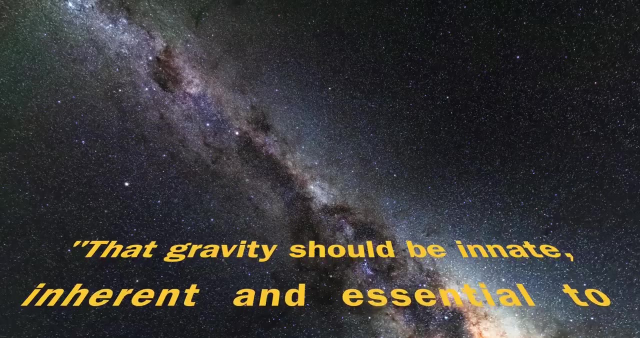 Get up to three months free, and if you're not satisfied in the first 30 days, you can cancel without paying a penny. Now onto my techie test question. Which famous scientist criticized Newtonian gravity by saying that gravity should be innate, inherent and essential to matter, so that one body may act upon another at a distance? 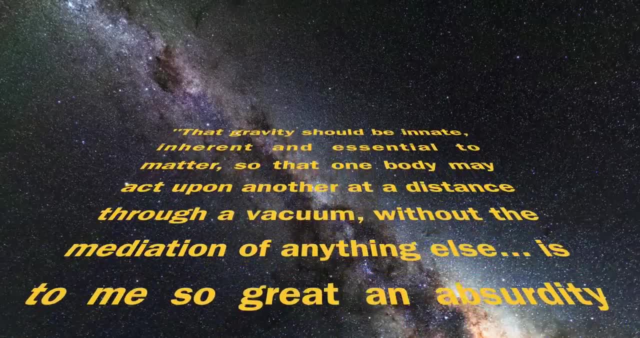 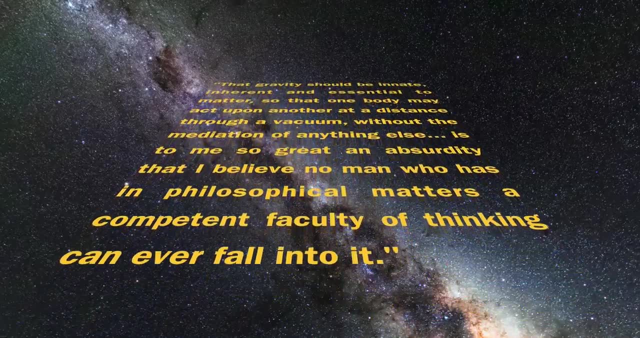 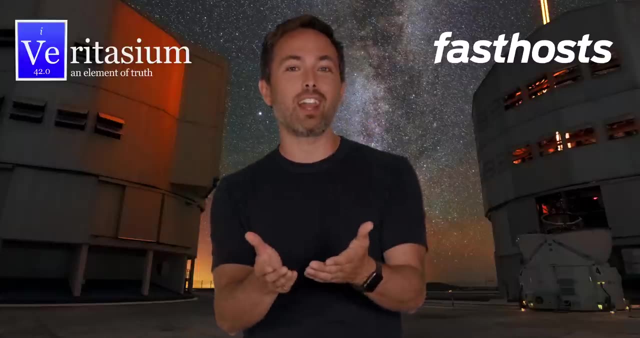 through a vacuum without the mediation of anything else. This is an absolutely so great an absurdity that I believe no man who has, in philosophical matters, a competent faculty of thinking can ever fall into it. If you know the answer, who said that? and you live in the UK? click the link below for. 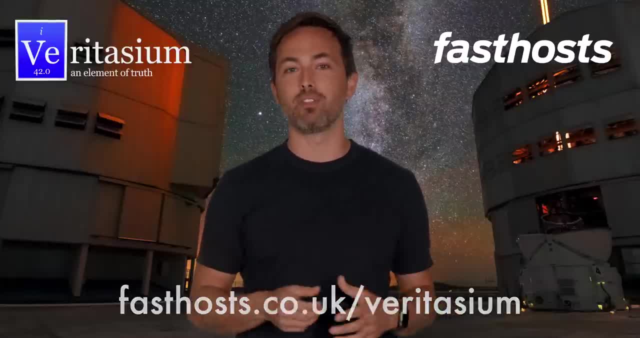 your chance to win the ultimate tech bundle. I want to thank Fasthosts for sponsoring this video and I want to thank you for watching.